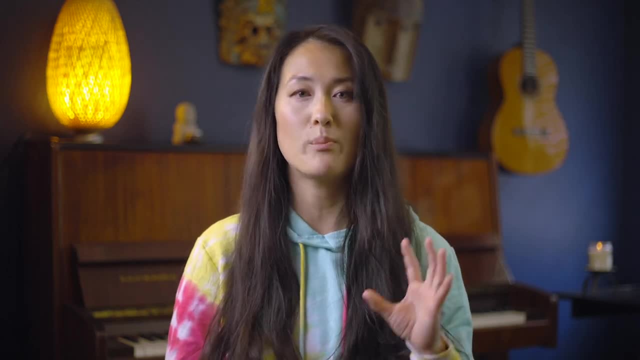 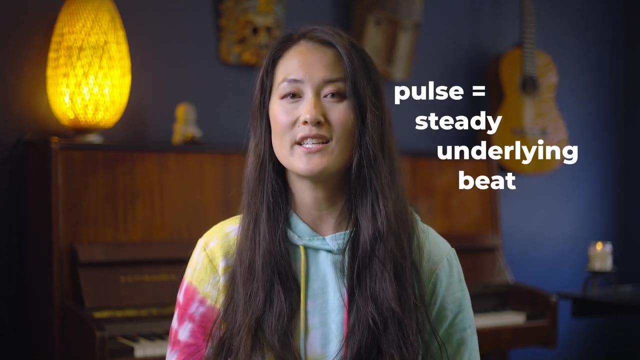 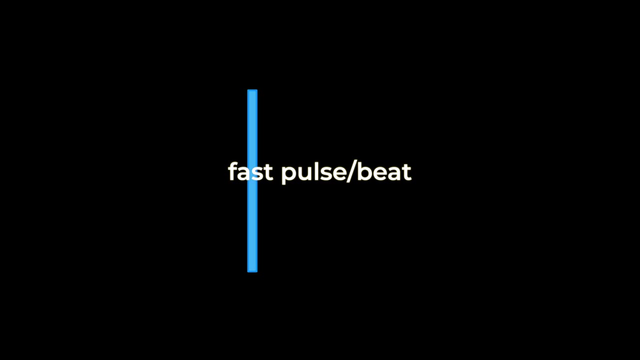 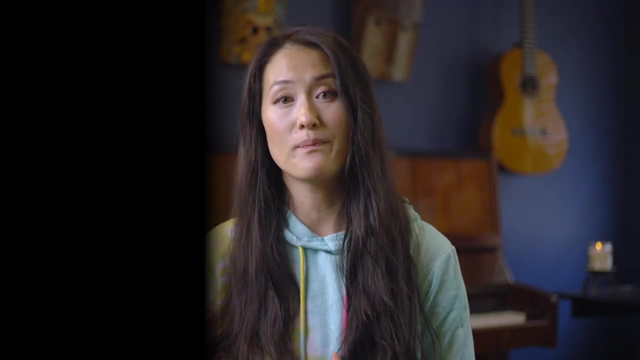 to the music. you're most likely doing that to the pulse of the song. The pulse is the steady underlying beat of the music that continues throughout. Sometimes the pulse or beat is fast and sometimes it's slow, But not to make someone glad. you never liaise. 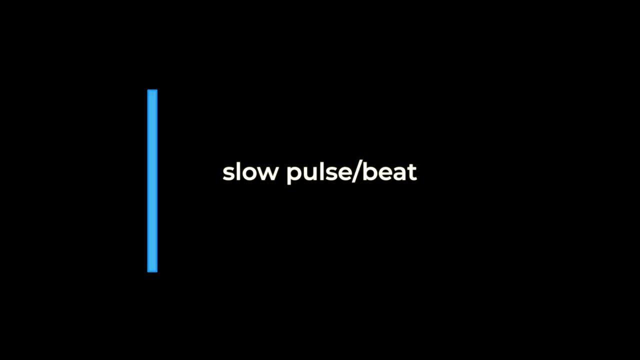 because usually when you listen to the notes you are happening to be having those sound papa-tas. It's a little bit harder and it feels amazing And you can essentially click the notes off easily if you'll just enjoy the rhythm, that works. 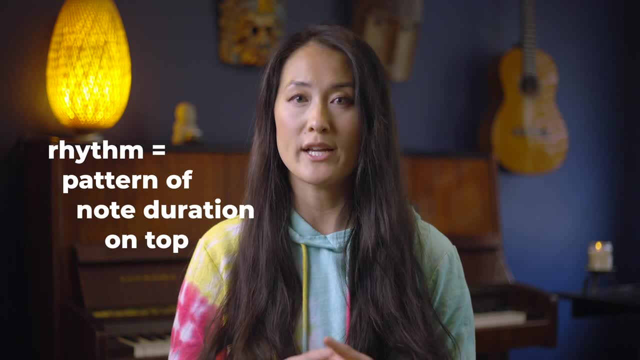 Now rhythm is the pattern of note direction you have to into an orderly pattern. You can pick patterns with theuden, though rhythm is me, you want to Holland. stick to those patterns by marvelous tricking. I've read recently where there were literally four or five. 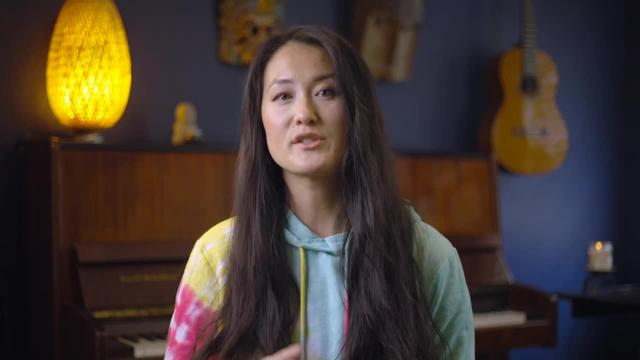 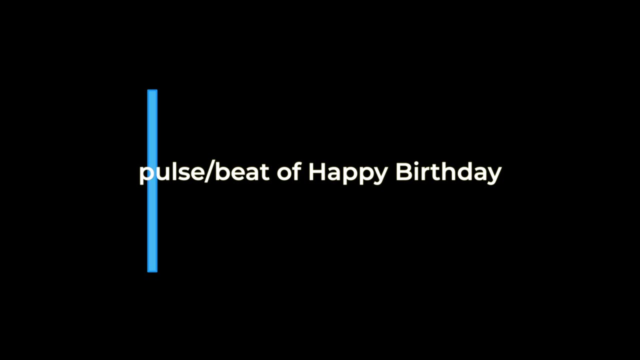 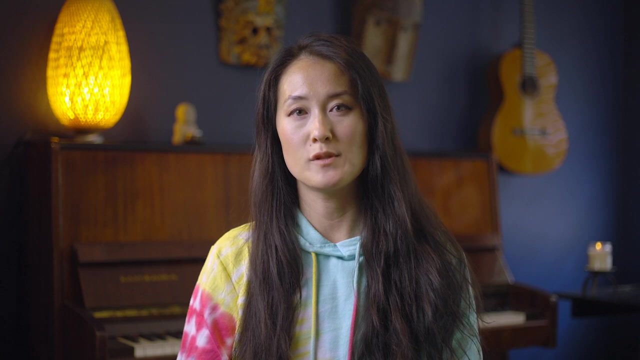 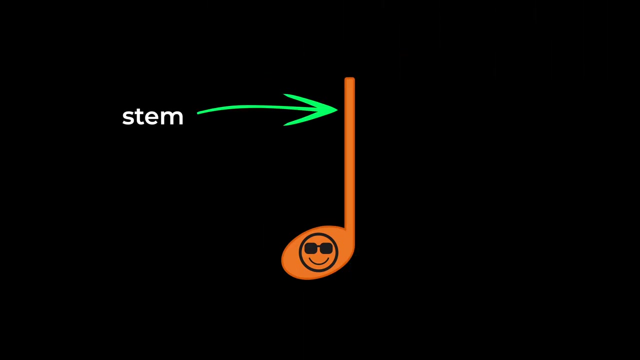 bars that I can play little projections of patterns. The truth is, if you're really playing a song on top of that steady pulse. So here's the pulse of happy birthday and here's the rhythm on top. So let's talk about note values. You remember our note head? right Now let's add a stem. 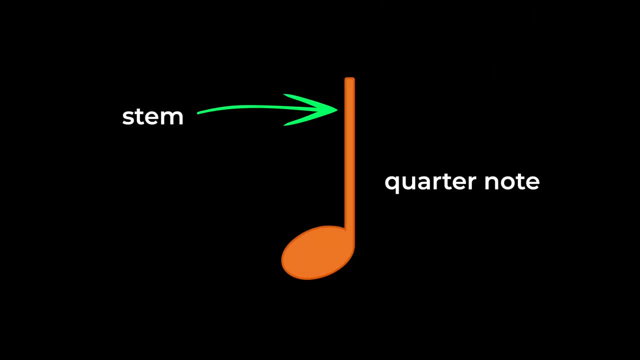 Notes that look like this last for one beat and are called quarter notes. So if I get my steady pulse going again, I can add a quarter note. So if I get my steady pulse going again, I can add a quarter note. So if I get my steady 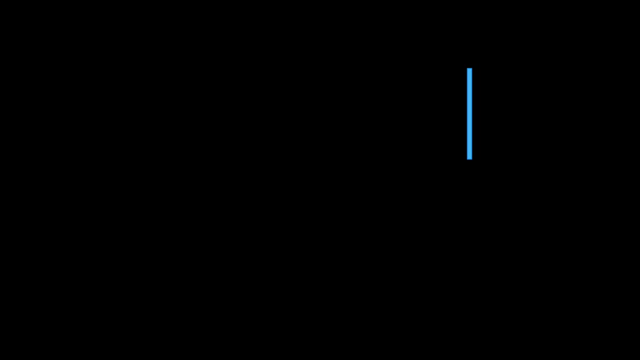 pulse going again, I can add a quarter note. So if I get my steady pulse going again and I see four quarter notes, I'd play a note for each quarter note and count one. I'd play a note for each quarter note and count one. 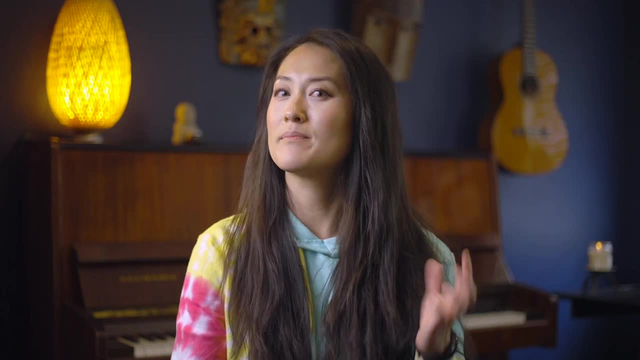 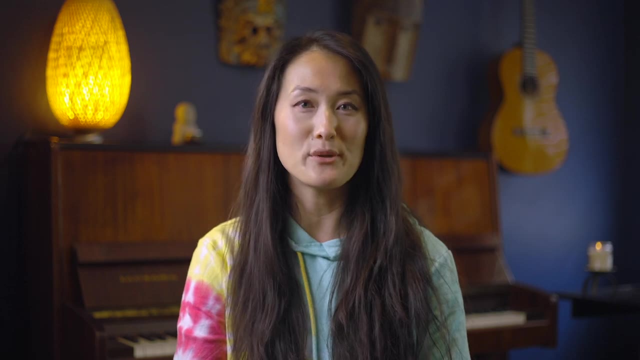 Now, when we see quarter notes, it's tempting to just think, oh, that gets one beat And simply count 1.. Well, yes, that's kind of the right way to do it. It is not complete without also having your steady pulse in mind. 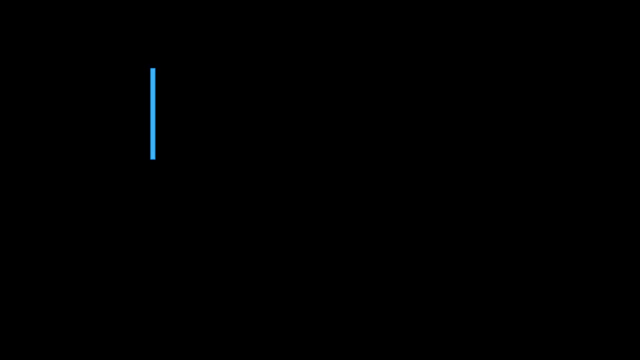 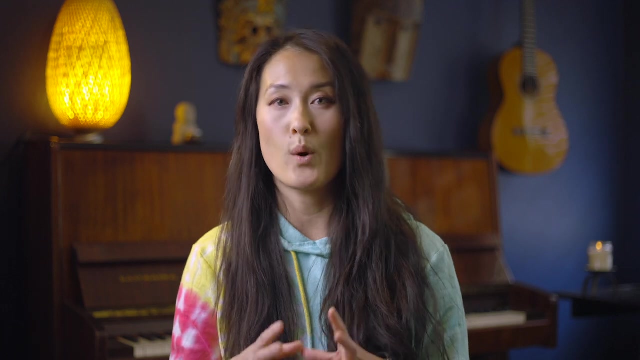 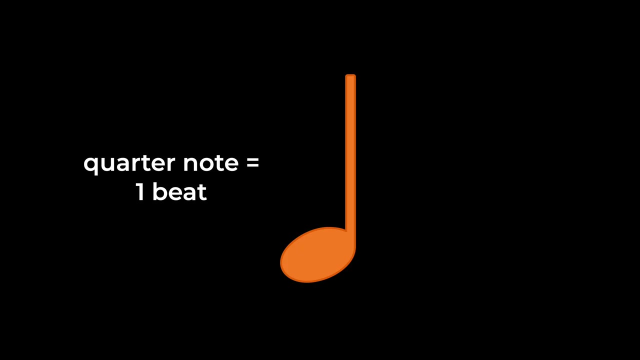 Because a 1 in a slow pulse will last a lot longer than a 1 in a quick pulse. If I erase the center of the note head, we get a half note which lasts for 2 counts or beats. And if I erase the stem, we get a whole note which gets 4 beats. 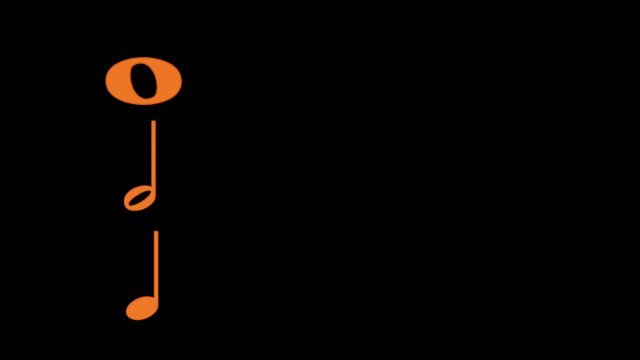 Working backwards we can see that these note value names make sense. If a whole note gets 4 beats, then a half note- or half of 4, would get 2 beats, And a quarter of a whole note is 1.. 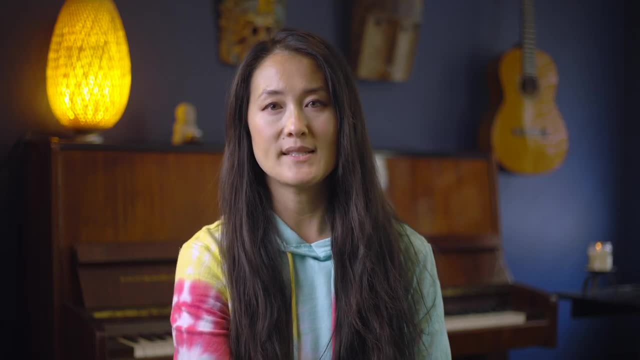 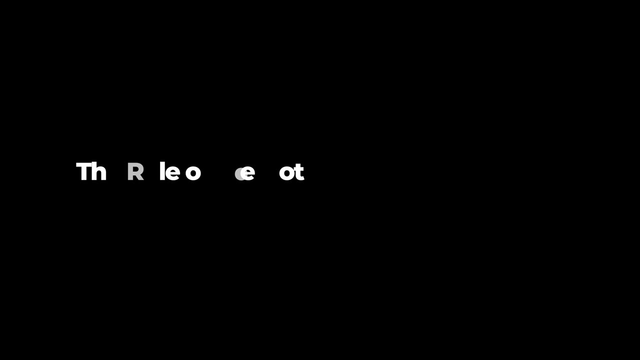 Now there's one more note value I want you to remember. It's actually not a value but a rule. I call it the rule of the dot. You can think of the dot as an addition sign. Any time we put a dot to the right of a note head. 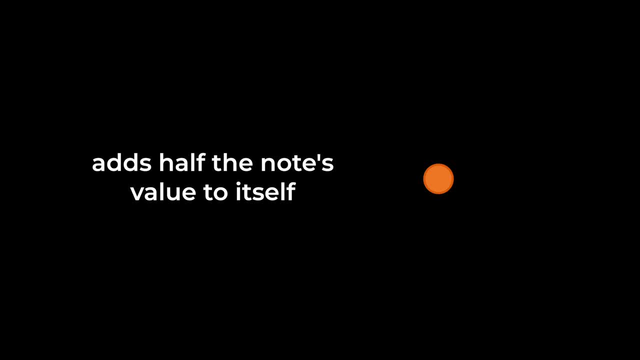 it automatically adds half of the note's value to itself. For example, here I have a half note which we know gets 2 beats. Now I'm going to add a dot to the right, so I need to add half of 2, which is 1,. 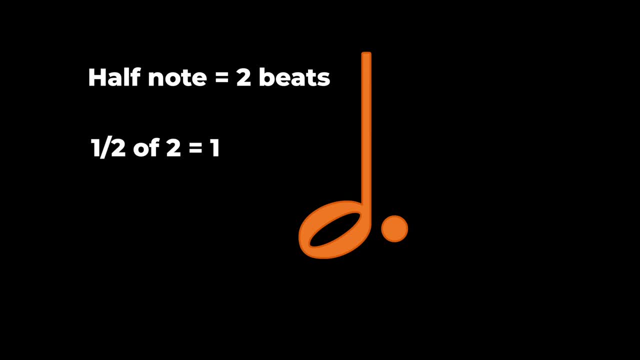 to the 2 beats that are already there. So we get 3, because 2 plus 1 equals 3.. And we call this a dotted half note. If we added a dot to the whole note to make a dotted whole note, how many beats would that get? 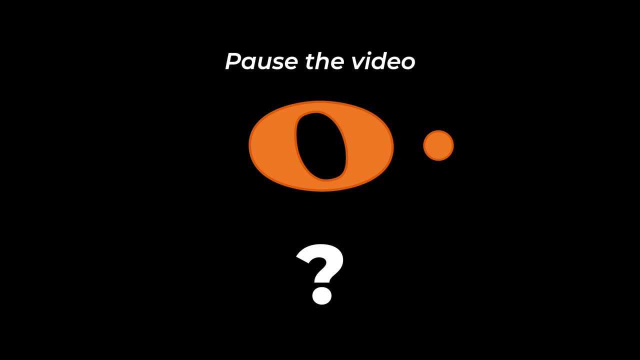 Pause the video if you want to think about it before we work through the answer together. So we know that a whole note gets 4 counts. Once we add the dot, we know we will be adding half of its value to itself. Half of 4 is 2, so 4 plus 2, or a whole note plus the dot. 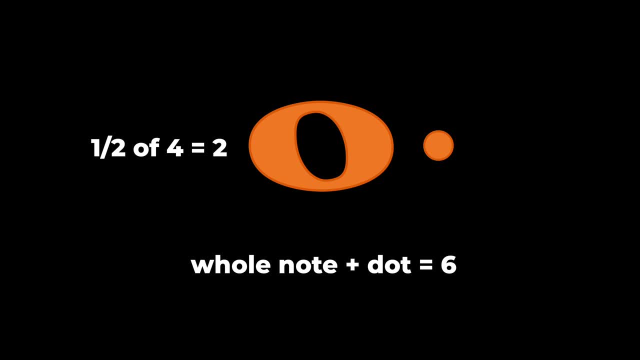 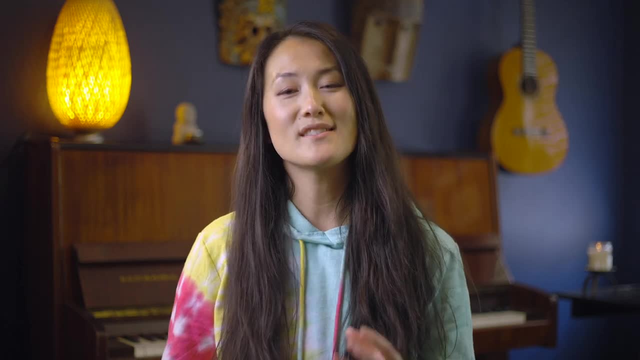 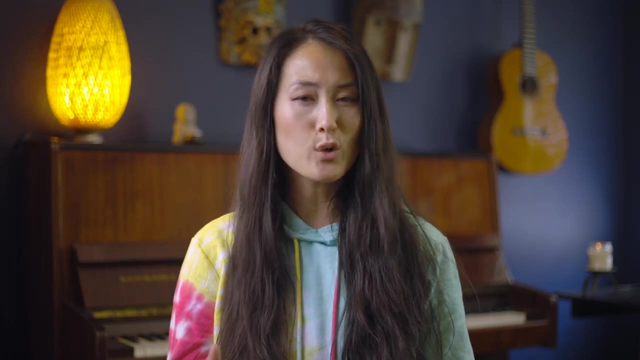 And that's the rule of the dot. Now it seems like music should only be audible sound, right, But silence is actually an important part as well. Silence can create drama, tension, awkwardness, and it can help give melodies some personality. 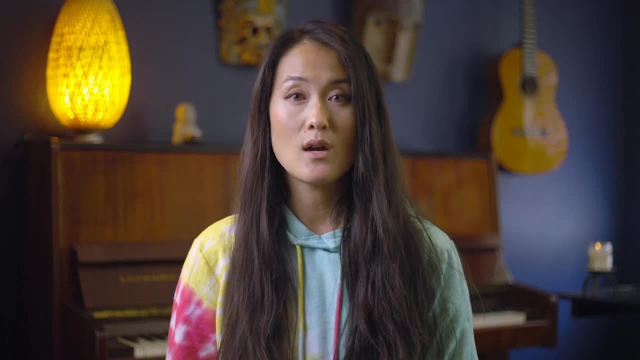 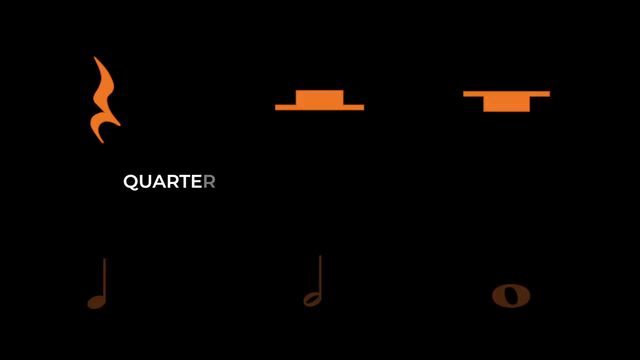 These silences are marked in sheet music with rests. Rest values are named and counted just like our other note values. A quarter rest gets 1 beat of silence, A half rest gets 2. And a whole rest usually gets 4 beats. 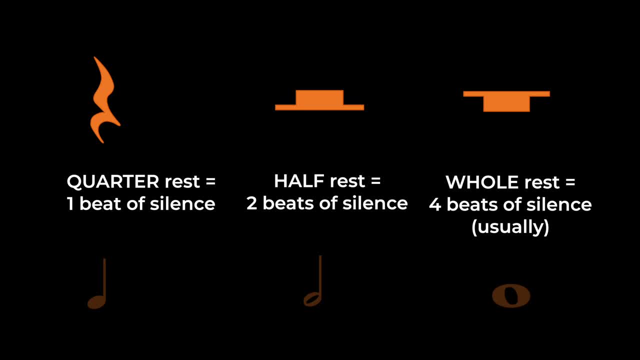 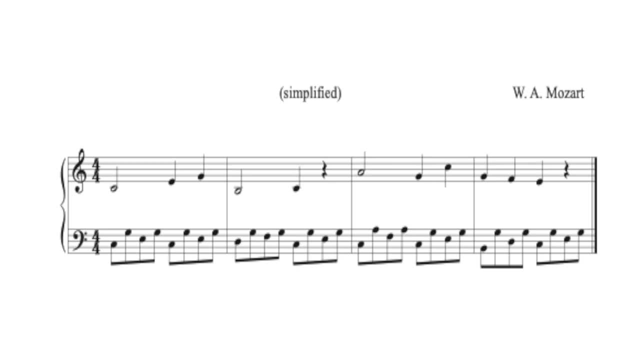 I said it usually gets 4 beats because there are exceptions to the whole rest and we'll talk about those in a minute. Let's look at Mozart's Sonata in C major, And we're going to take a minute to identify everything we've learned so far. 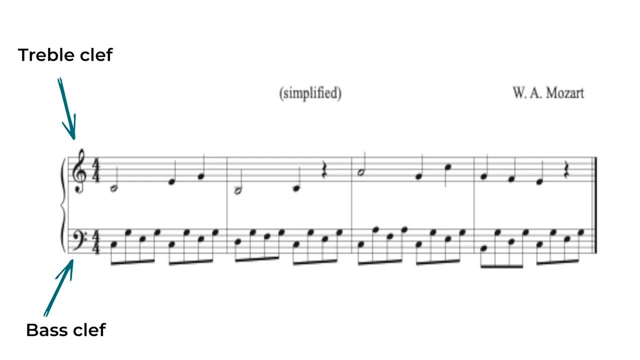 We've got the treble clef and bass clef, The grand staff connected together with this squiggly line or brace, And we have note heads and stems. Now do you recognize any of our three important notes that we learned at your last lesson? 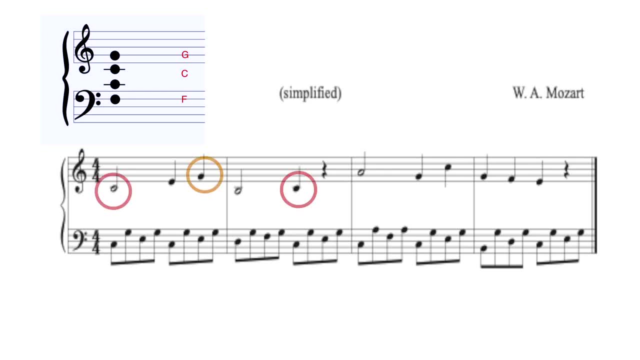 I see middle C's, Treble G's And bass F's, And we just learned that these are quarter notes and these are half notes And we know that these right here are quarter rests. So we already know quite a lot. Now let's check out these lines here. 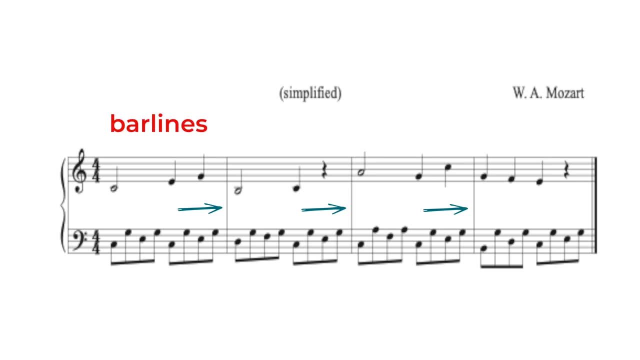 These are called bar lines and they separate notes into nice and neat measures. There are four measures Now look at this. This is called the time signature and it's found at the beginning of pieces. When we refer to it, we say four, four time. 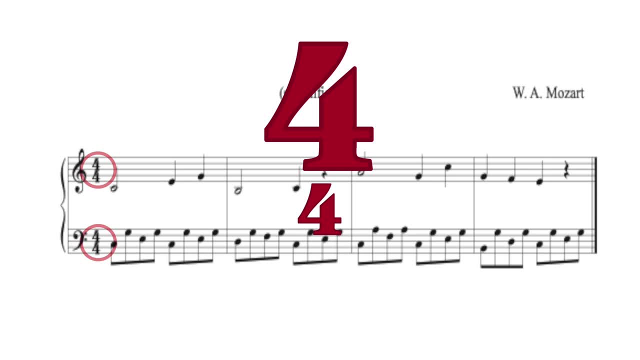 The top number tells us that in every single measure there are four beats. If we look at the first measure here and add up the note values in the right hand, we can see that they do add up to four, because a half note plus two quarter notes equals four beats. 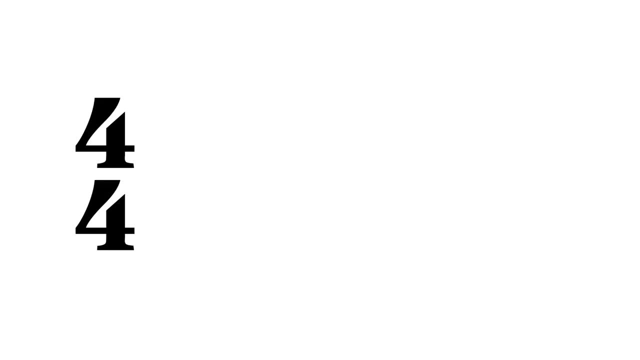 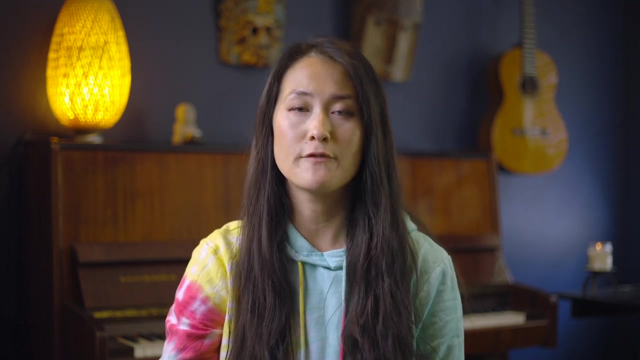 Same with the second measure. So now that we know what a time signature is, instead of just counting 1, 1, 1, 1 for four quarter notes, we count 1, 2, 3, 4 for every measure. Okay, let's try some other rhythms in four, four time. 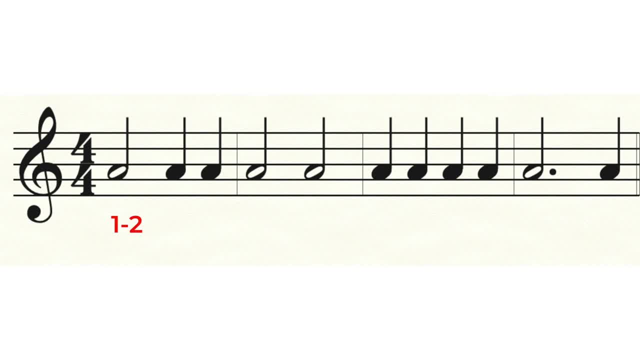 First I'm going to write in the counts: 4: 4 time: 1 1 1 1 1. 4 4 time: 1 1 1 1 1 1 1. 4 quarter notes: 4: 4 quarter notes. Okay, let's try some other rhythms in 4- 4 time. I'm first going to write in the counts: 1, 2, 3, 4 for every measure: 4- 4 time: 1 1 1. 1, 1, 1 for every measure 4- 4 time. 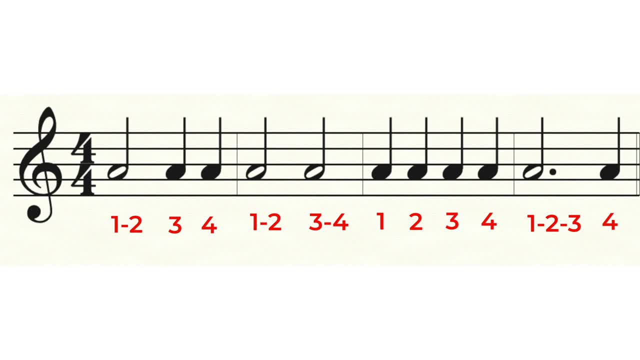 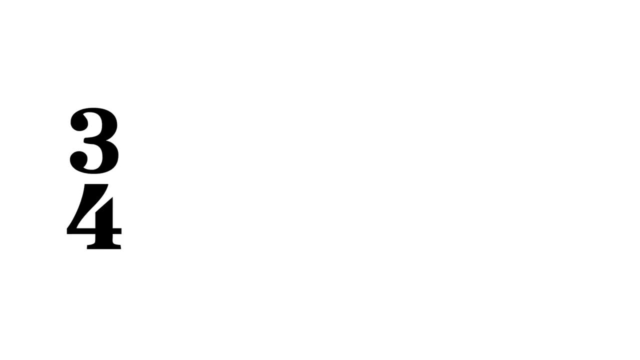 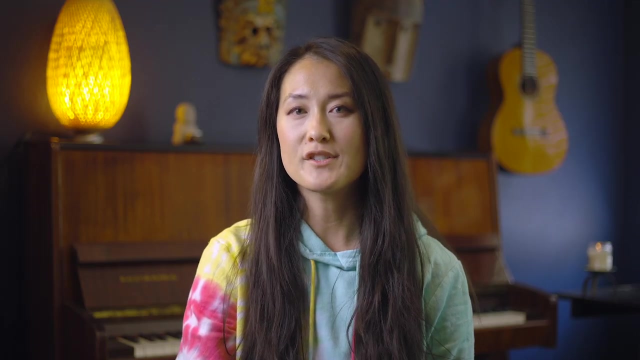 Good, Now what if we saw this? Remember, it's the top number that we're concerned about. This three tells us that there are three beats in every measure. So we count one, two, three, One, two, three And we feel a nice strong beat: one, Two quick side notes. First I told you the 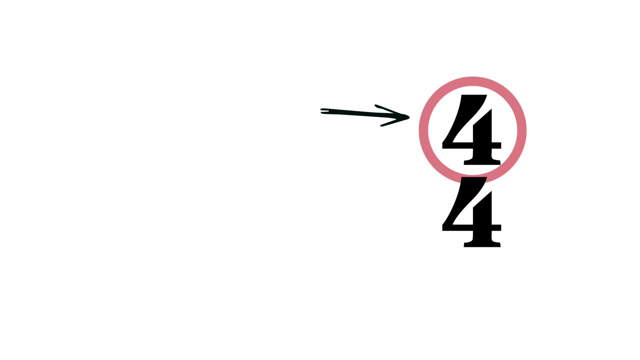 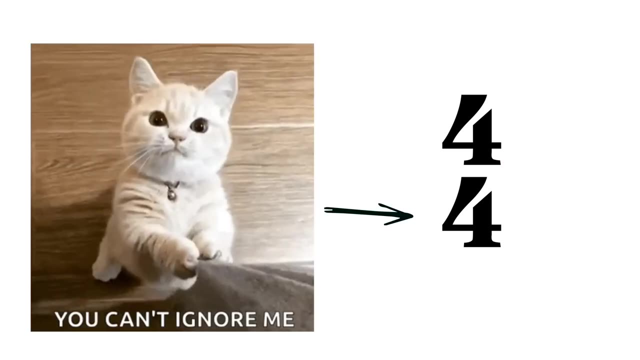 top number of the time signature tells us how many beats we've heard in the last several seconds. So if you count one, two, three, four, One, two, three, four are in each measure The bottom number has a different function, but for now we're just going to ignore it. 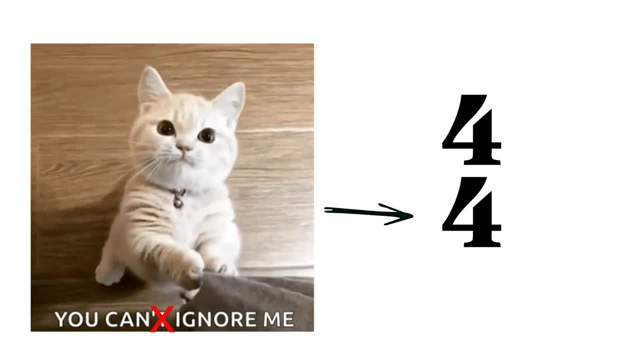 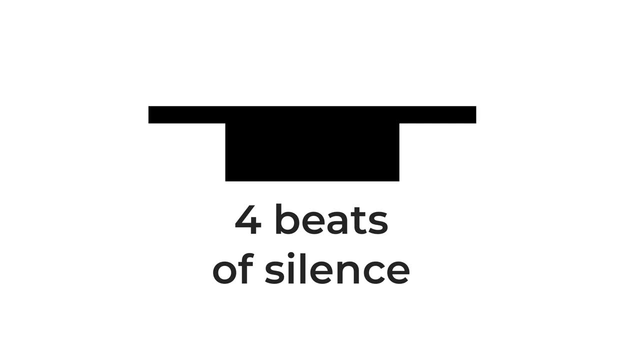 as it's not yet important for us to know. And second, I mentioned that usually the whole rest gets four beats of rest, with some exceptions. Now that you know about time, signatures and measures, I can tell you the real value of a whole rest is a whole measure of rest. 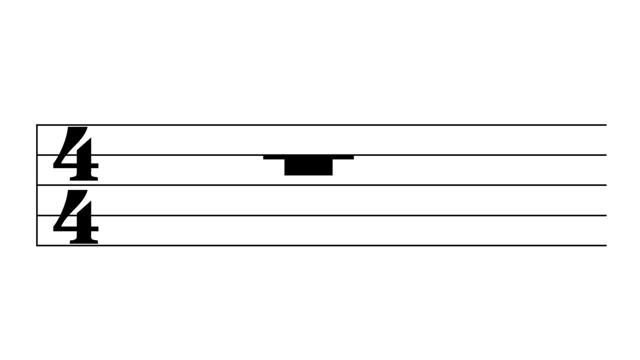 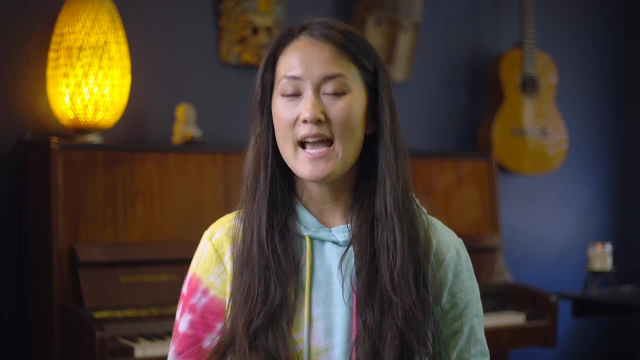 So if you're in 4-4 time, a whole measure of rest will be four beats, But if you're in 3-4 time, a whole measure of rest will only be three beats. Let's test your ear. I'm going to play some tunes and let's see if you can tell whether they're in 4-4 time. 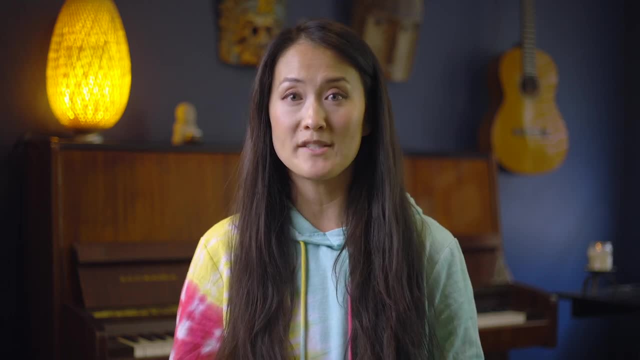 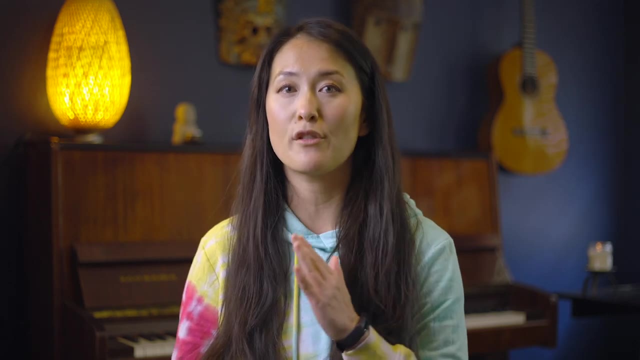 or 3-4 time- And I'm going to exaggerate this strongly Strong beats a bit. So in 3-4 time, beat 1 is strong and in 4-4 time, beats 1 and 3 feel strong, with 1 being. 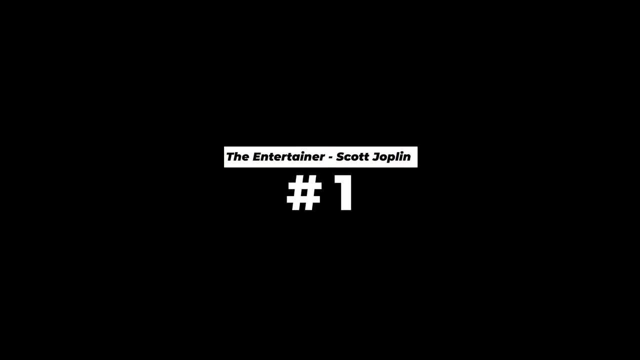 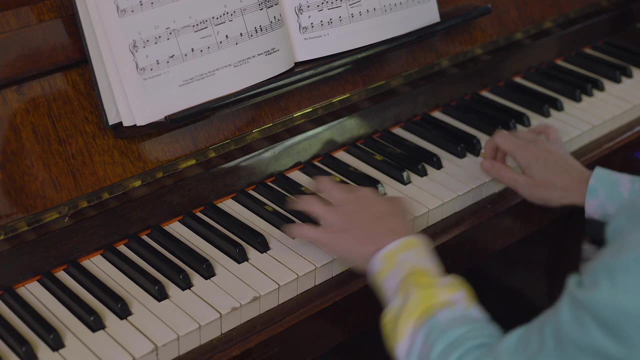 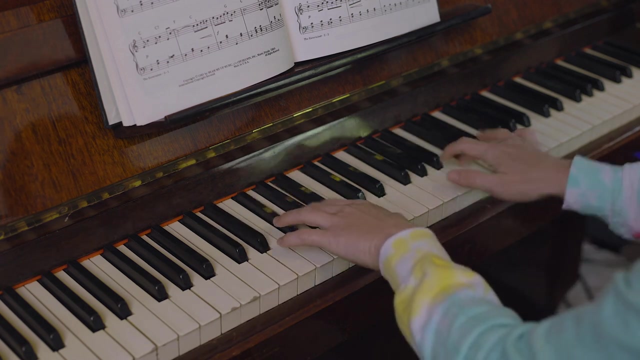 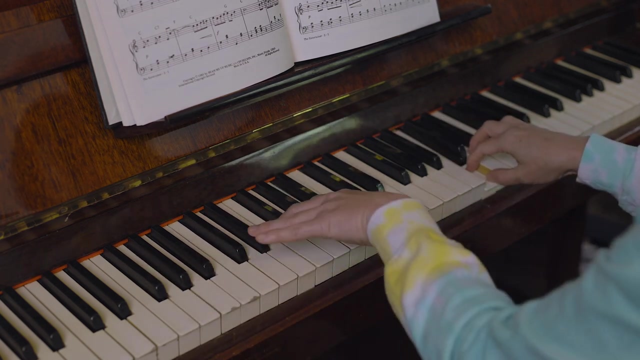 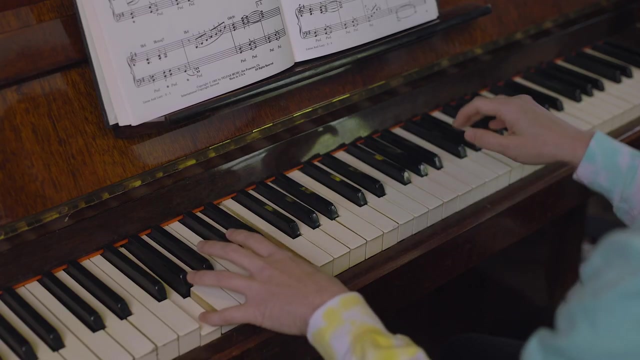 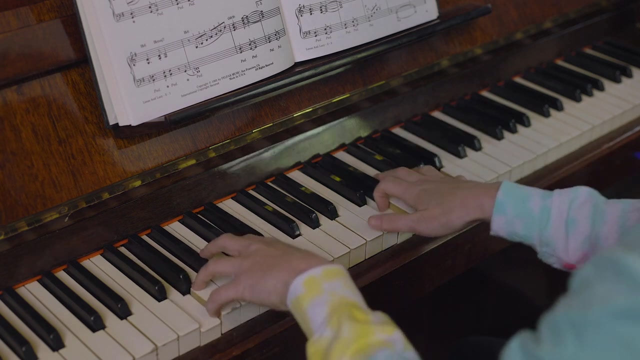 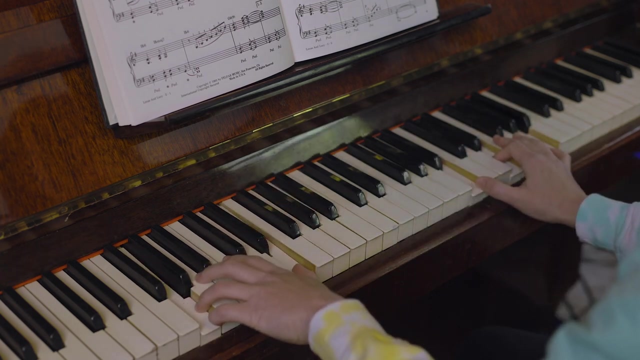 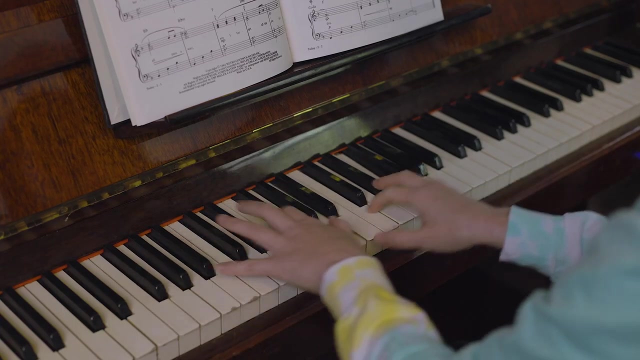 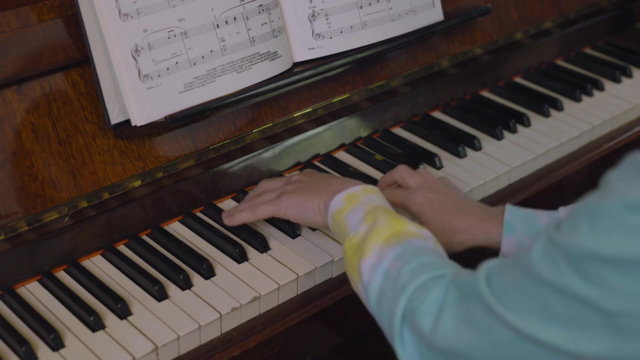 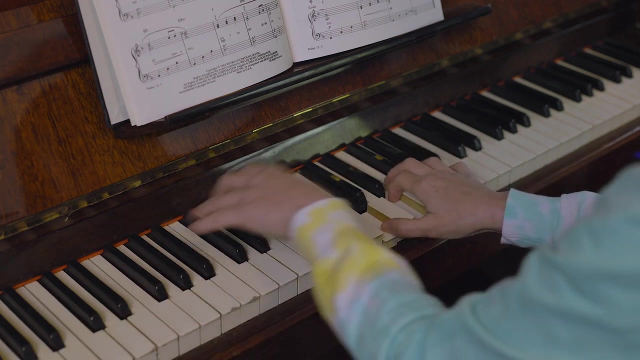 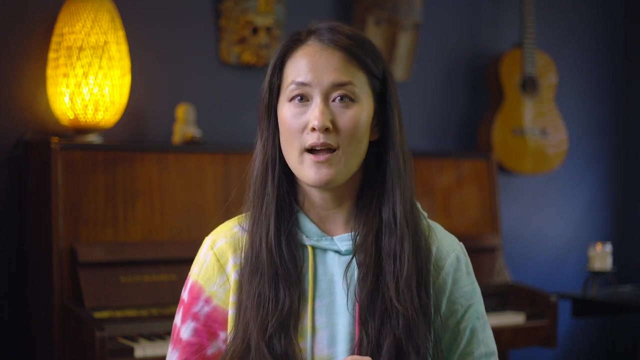 the strongest. Basically, the whole thing Good. Uh-huh Good. How do you feel now? Uh-huh Review Sounds smaller, 2-0.. Before you give me your answers, I want you to listen to them one more time and count. 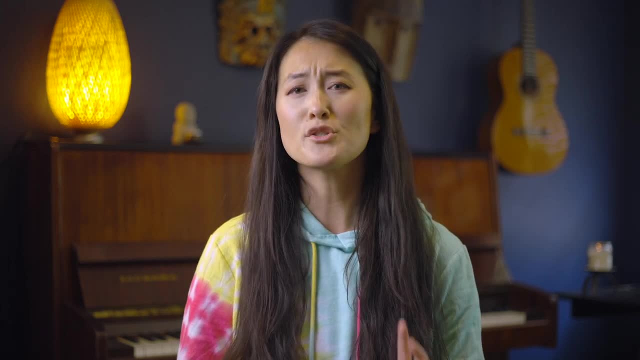 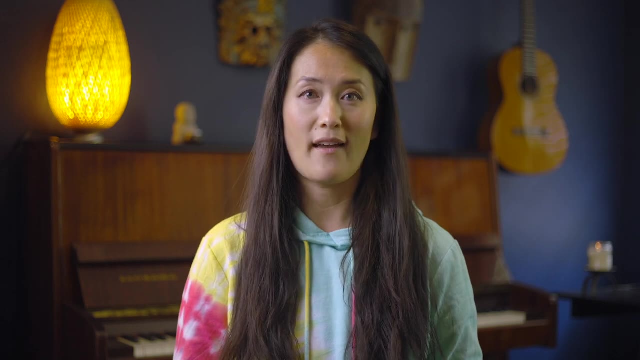 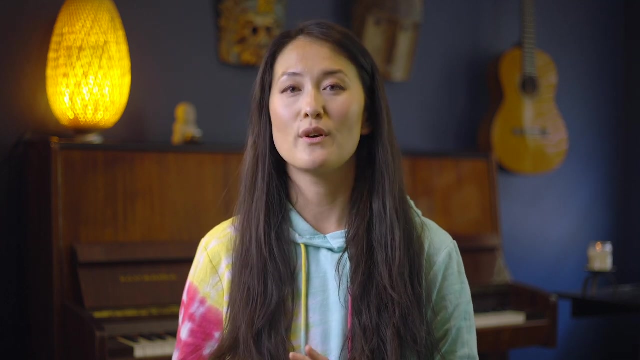 in whatever time signature you think it is. So if you think it's in 3-4 time, you'll count 1, 2, 3,, 1,, 2, 3.. And if you think it's in 4-4 time, you'll count 1,, 2,, 3, 4,, 1,, 2,, 3, 4.. 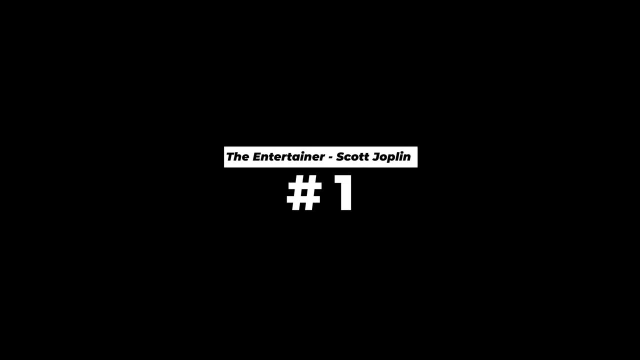 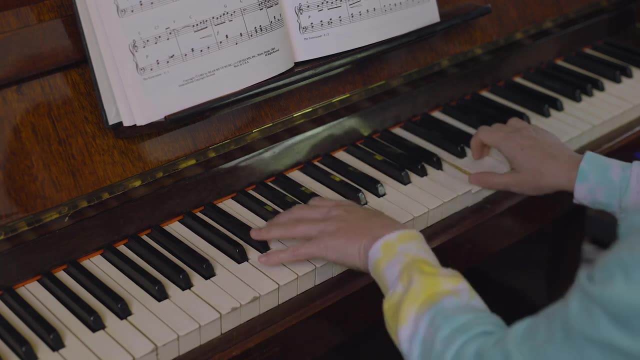 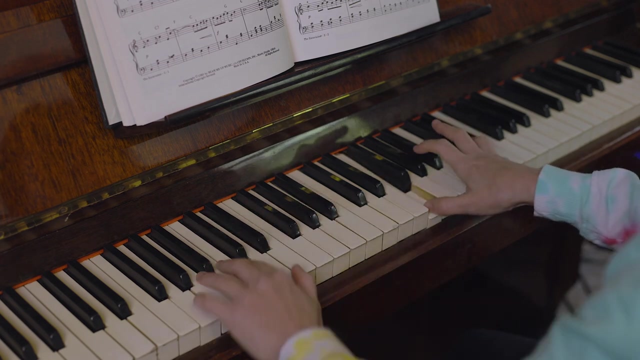 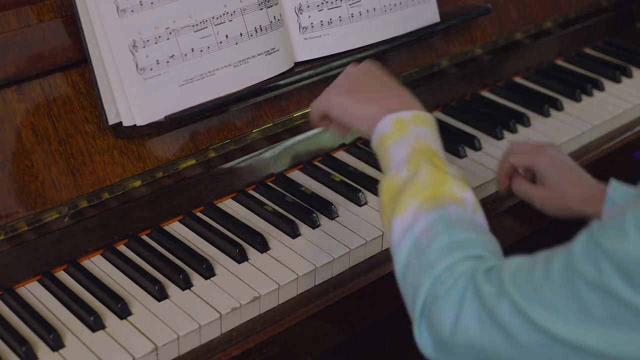 Okay, let's hear them again Now. the first answer is 2, 2, 3, 1, 2, 3, 4.. Okay, so you'll count another 2-3 times, All right? 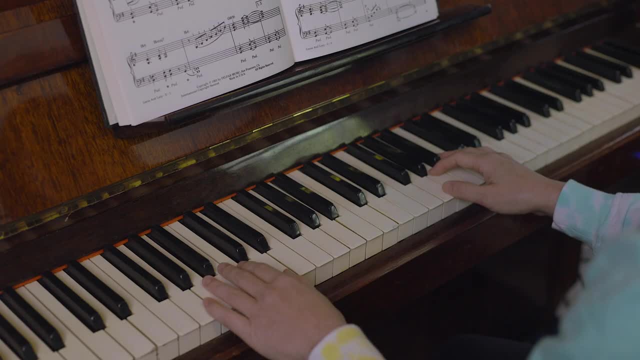 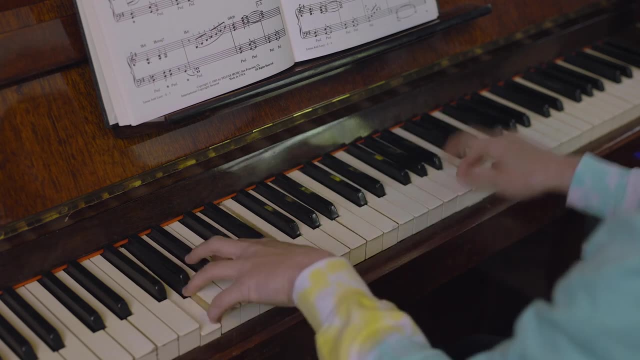 So you're going to count them one by one. So we'll start with this one. So here's one. We're going to count 2-3 times: 1-3, 2-3, 1-2, 3-4, 1-2, 3, 4, 1-2, 3-4, 1, 2-3, 1, 2-3.. 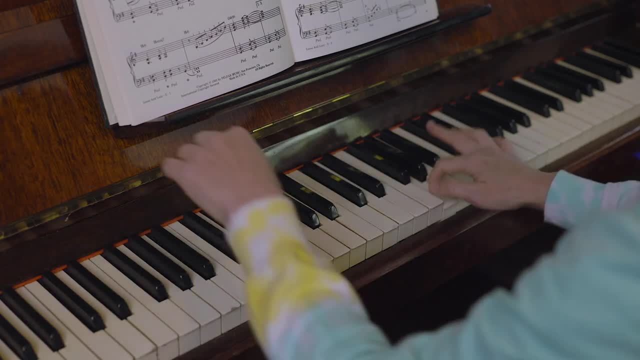 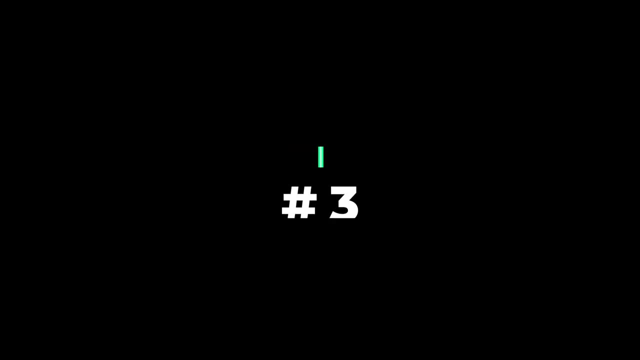 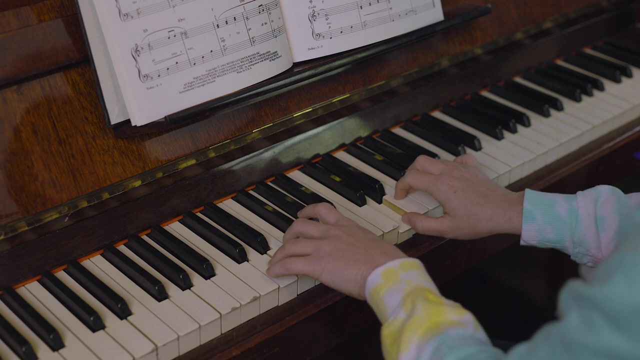 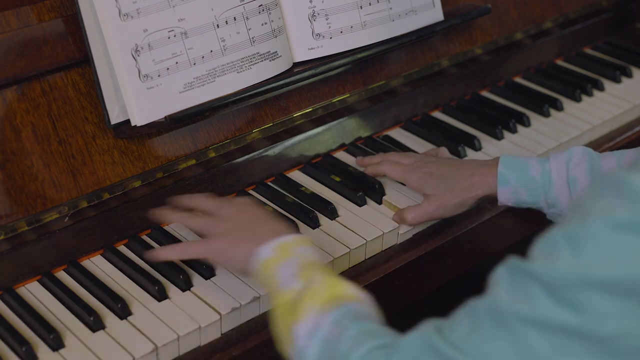 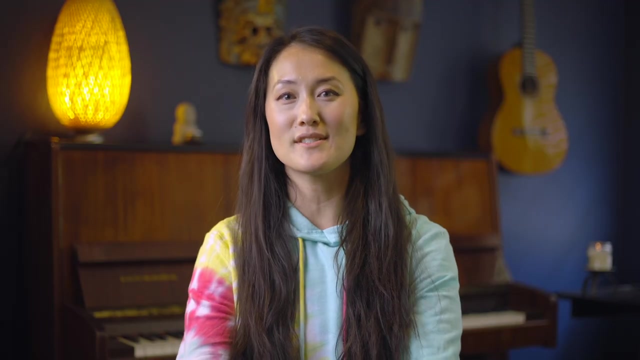 And here we have one 1-3 times. One One time 1-3 times, 1-3 times, 3 times 1-3 times 1-3 times. Alright, let's check out the answers. 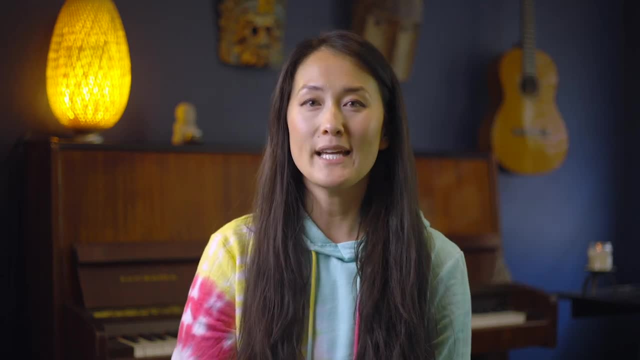 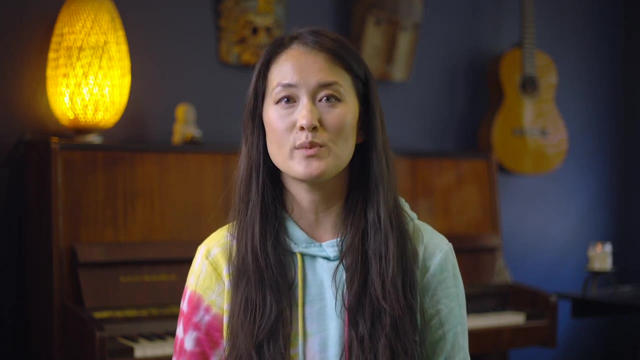 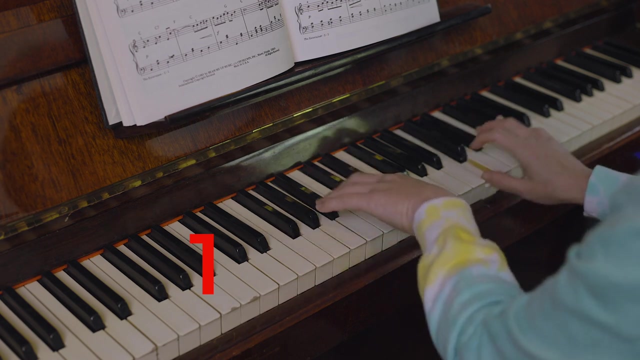 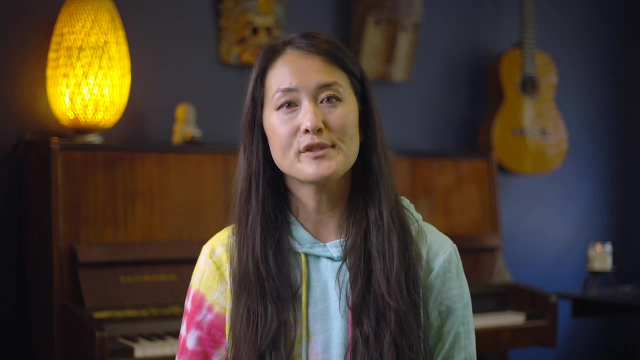 Number 1 was in 4-4 time. The right hand was kind of all over the place rhythmically, but the left hand was giving you a nice steady pulse with stronger beats on 1 and 3.. And number 2, which was Linus and Lucy, was also in 4-4 time. 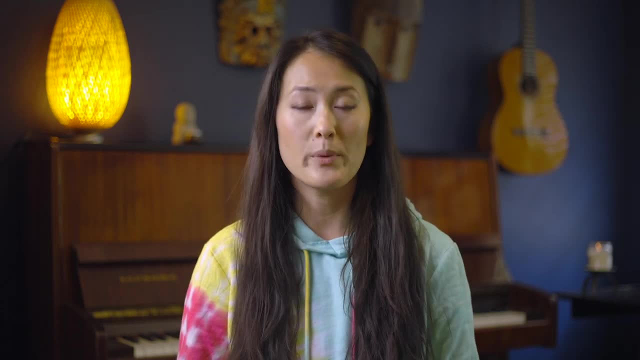 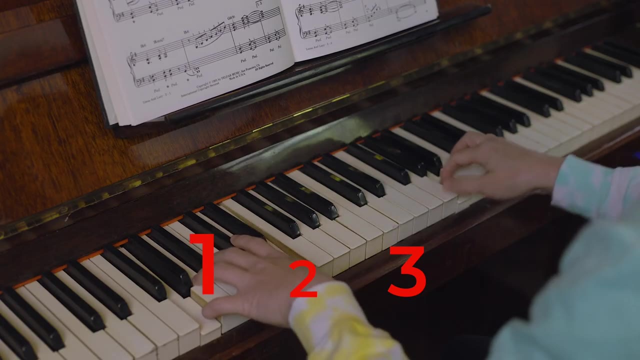 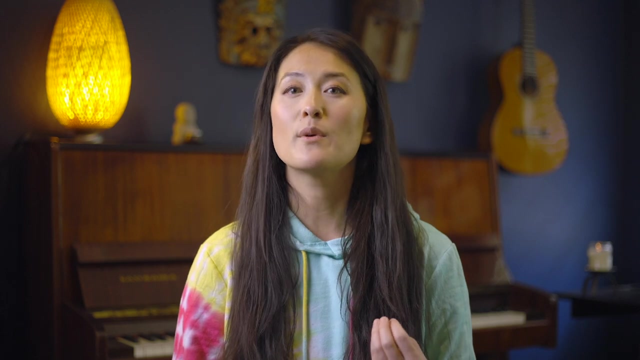 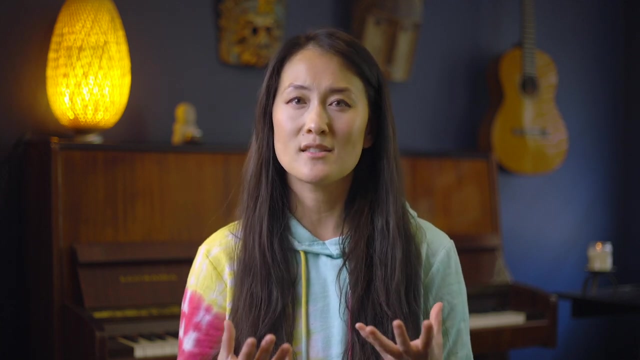 In this piece, though, the left hand was a little offbeat rhythmically, but the right hand was nice and solid, Especially on your strong beats 1 and 3.. And finally, number 3 was in 3-4 time. Even though this is a really gentle piece, could you sense the slightly stronger feel? 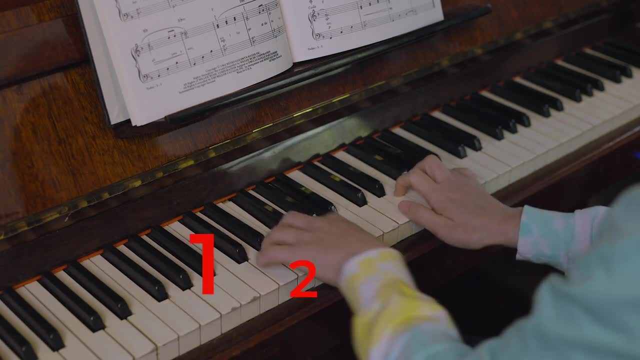 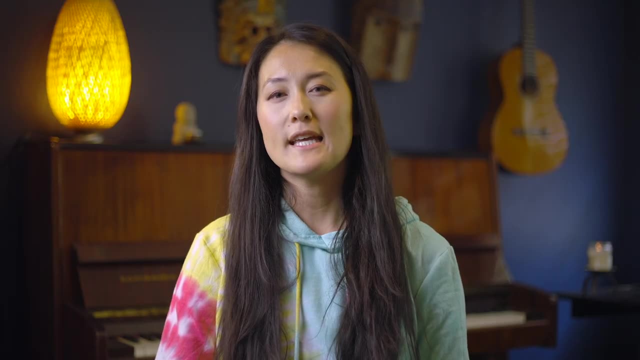 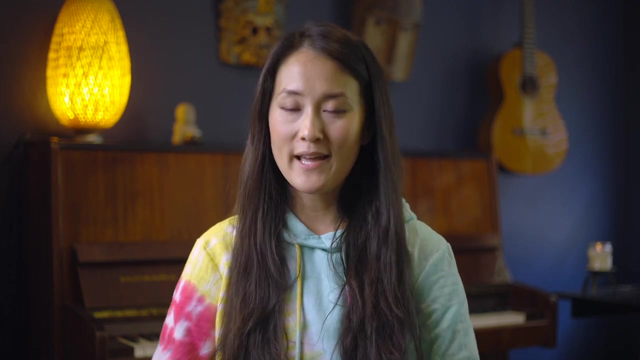 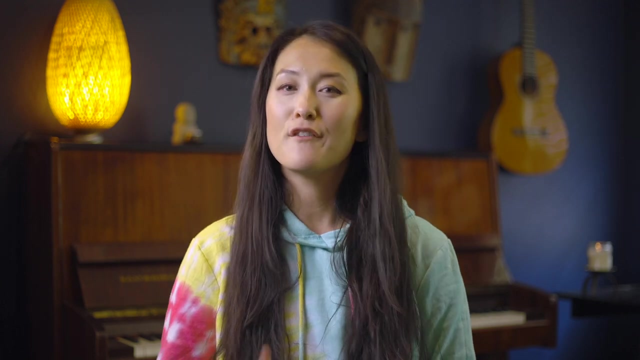 on beat 1?? If you had trouble picking out the time signatures, do not worry. The more you learn, play and consciously listen to music, the easier it'll be to pick out those types of things For your assignment. I want you to download the short practice exercises below: 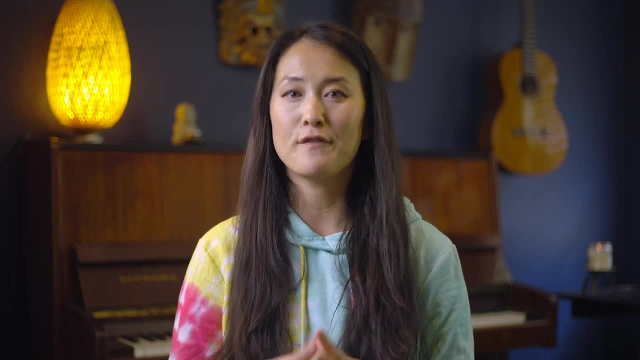 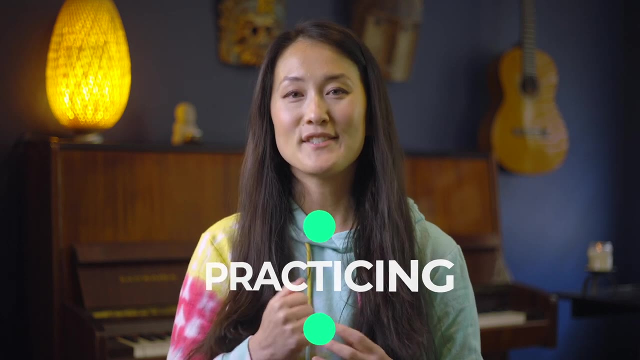 I've combined reading, music and rhythm on the grand staff for you to practice. Now let's quickly talk about practicing. So let's start with the first exercise, Number 1.. Some things that we learn in life. we only have to learn once. 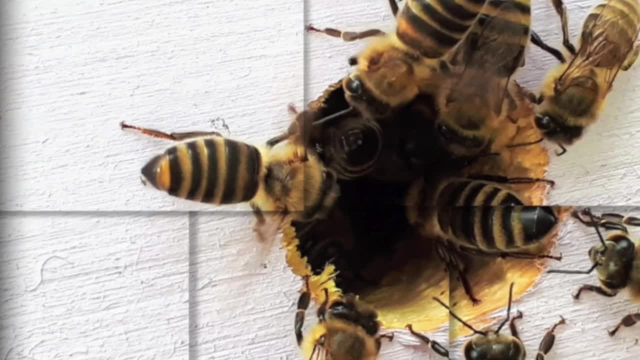 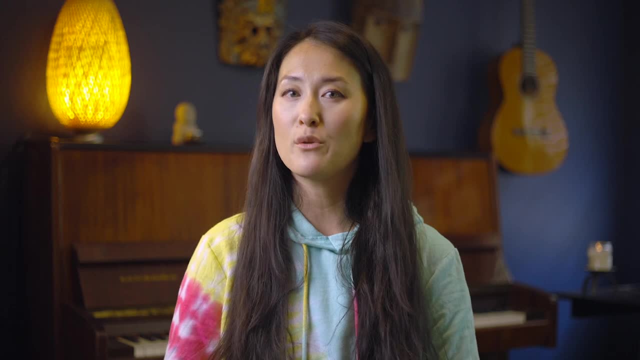 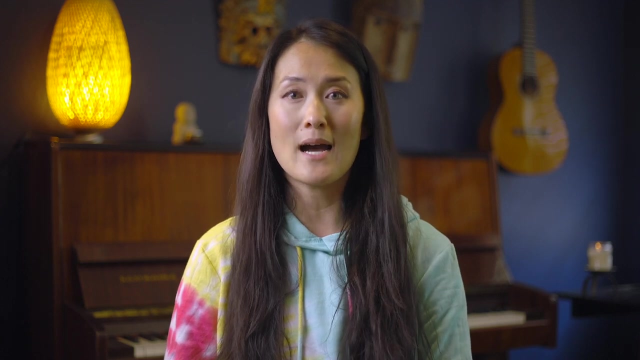 Like the fact that bee stings hurt, Avoid bees. But learning how to play the piano takes consistent practice. So if you play through these exercises once and think, oh, I'm done, you're not setting yourself up with the practice habits necessary to really see improvement. 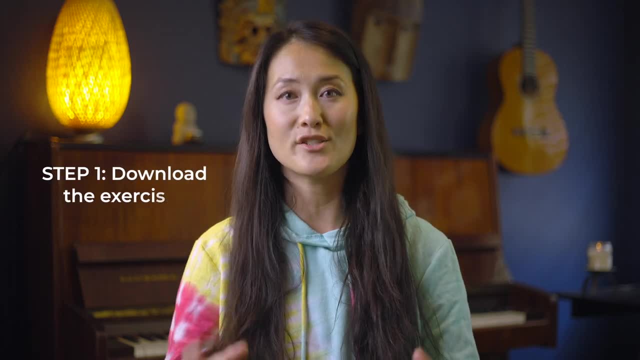 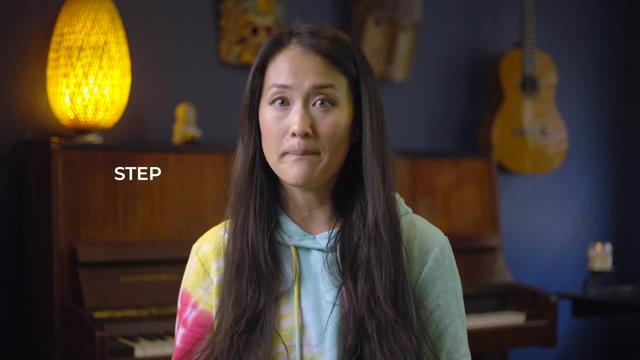 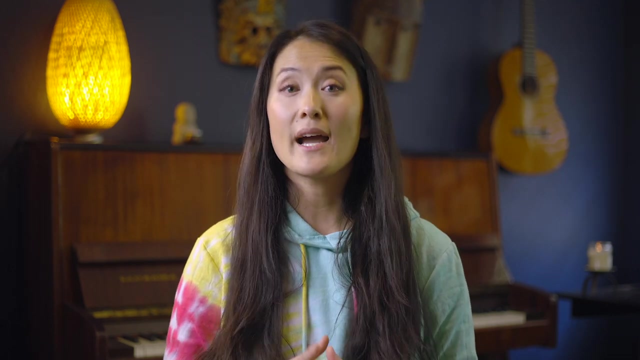 So ideally, you'll download these exercises and start practicing. Maybe you want to set a goal of practicing 5 days a week for 5 to 10 minutes a day. It's totally fine to start out with very small attainable goals. We're starting simple. 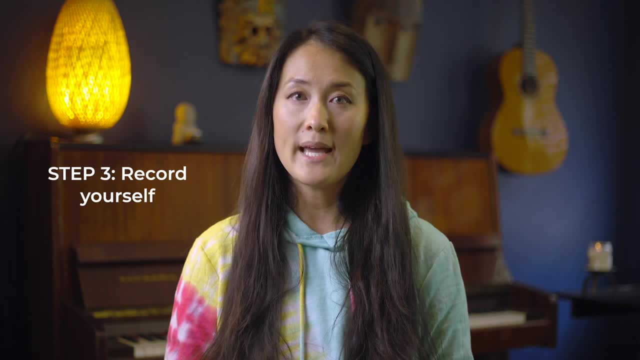 And I highly recommend recording yourself When you're playing. it can be difficult to really listen to how you're sounding because you're so focused on the action of playing, And when you listen back to your recording, I bet that you'll probably hear more mistakes.